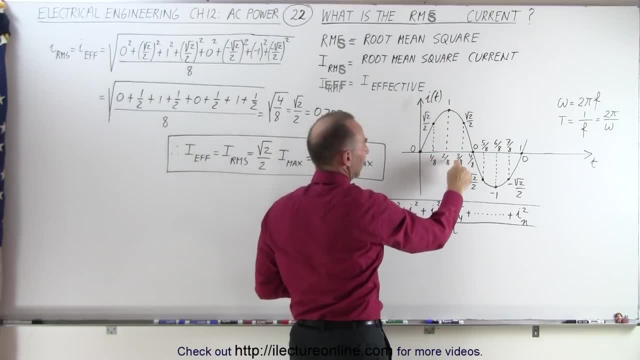 current is the square root of 2 over 2.. After 2- 8, it's 1.. After 3- 8, it's the square root of 2 over 2.. After 4, 8 or halfway through the period, we're back down to zero. Now we get the negative values. 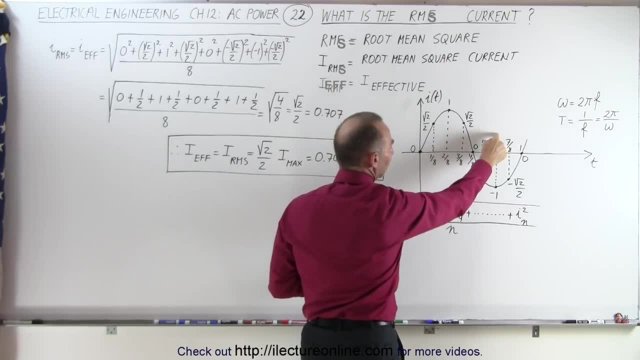 After 5- 8, it's minus the square root of 2 over 2.. After 6: 8, it's minus 1.. After 7: 8, it's minus the square root of 2 over 2.. And then again, if we then complete the whole period, 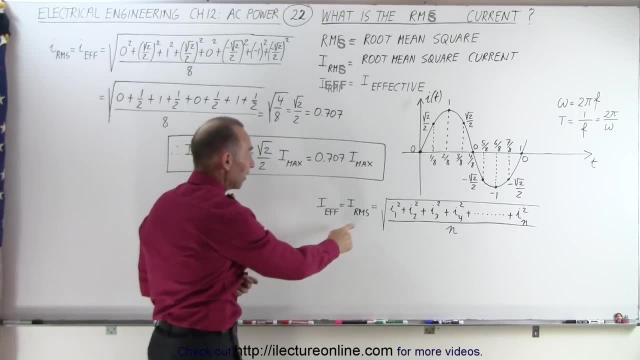 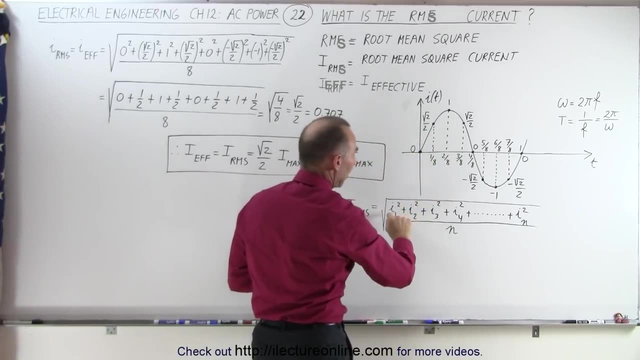 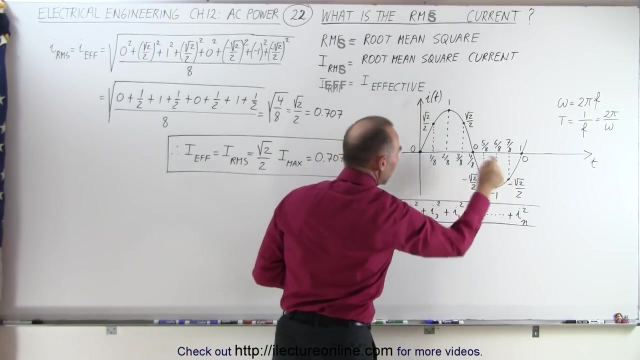 we get back to zero. By definition, the RMS current, or the effective current, is equal to the square root of the value of the current at each one of those intervals: I1. So we start with I1, over here I2, I3, I4, I5, I6, I7, I8.. We square those values, add them all up, then divide that by the total. 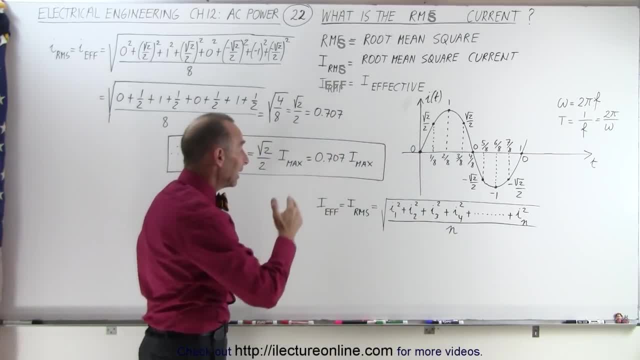 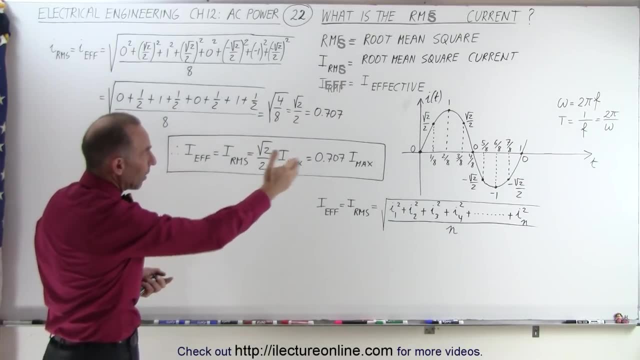 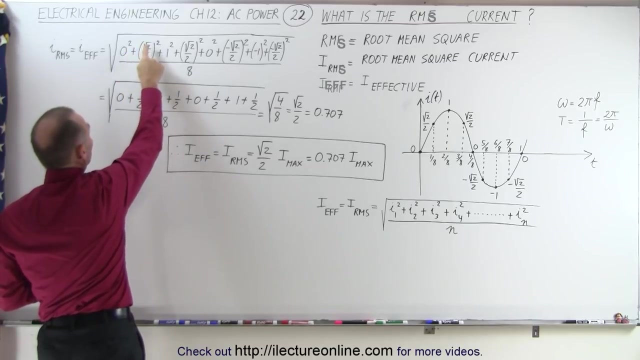 number of samples that we took, We square root of that and that then gives us the RMS current or the effective current that affected that equivalent DC current. So trying that with these eight values the effective or RMS current is equal to, it'll be 0 squared plus the square root of 2 over 2 squared plus 1 squared, and so 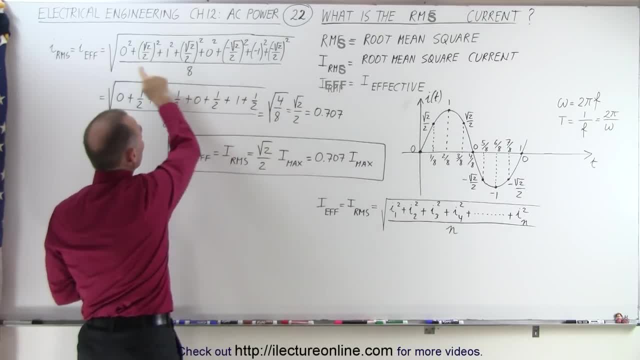 forth. We take all eight samples, We square the value of each, We divide it by the total number of points. That then becomes 0, 1 half, 1, 1 half, 0, 1 half, 1 and 1 half plus 1 half, So that 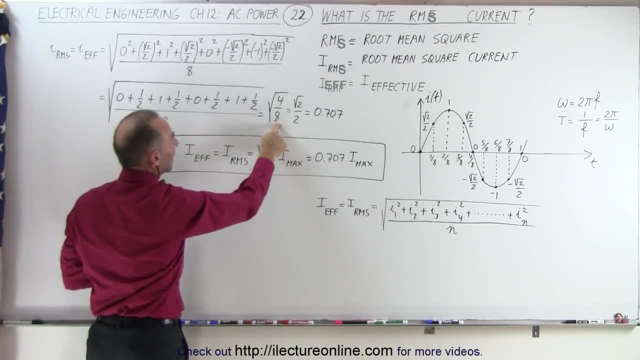 will be the eight sample points divided by eight. Sum them up: We get 4 over 8 or 1 half. Take the square root of that and we get the square root of the 2 over 2 or 0.707, which by now should be a. 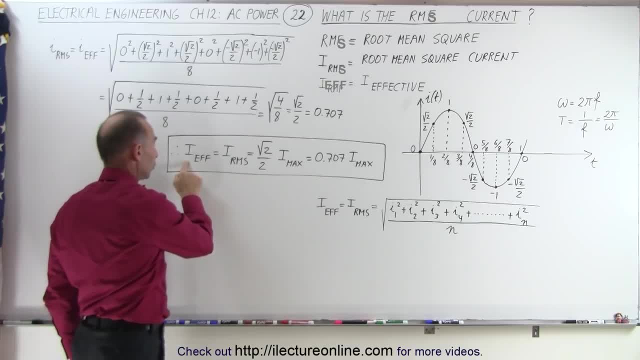 familiar value. So essentially the effective current or the root mean square current is equal to the square root of 2 over 2 times the maximum current. Remember in this example the maximum current was 1, but if the maximum current is 2 or 3 or 4, we simply multiply that. 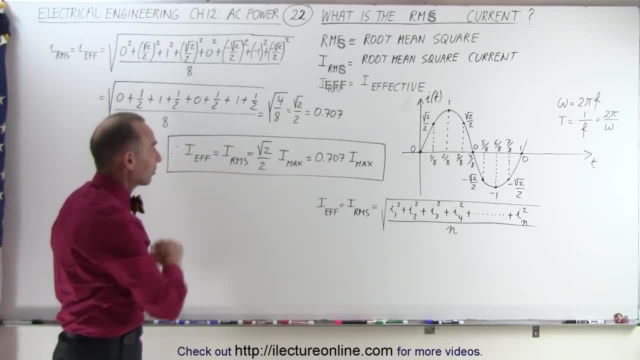 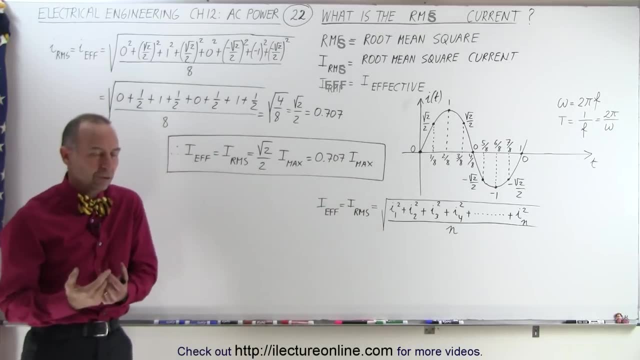 times, whatever that maximum current is. So in general we just call the maximum current times the square root of 2 over 2, or 0.707 times Imax, which is therefore the effective current. So we have an AC current, The equivalent effective current, in other words the equivalent DC current. 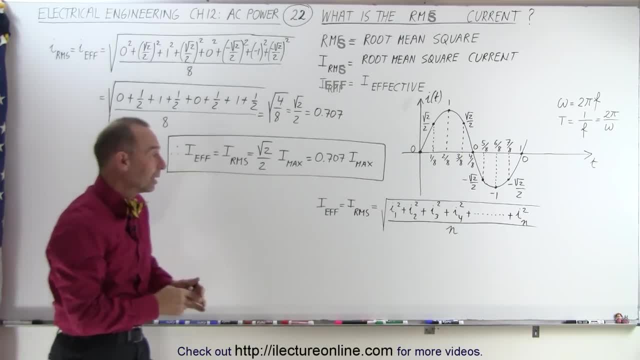 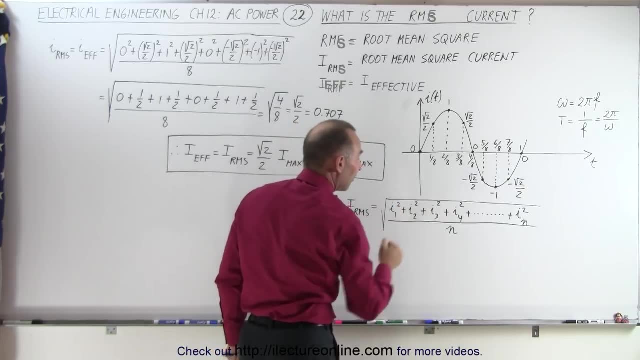 that will give us the same power delivered to the load can be calculated by using this formula, And that form is called the root mean square formula. We just take every value, We square every value, We divide it by the total, That's the average of the squares- And then we take the square. 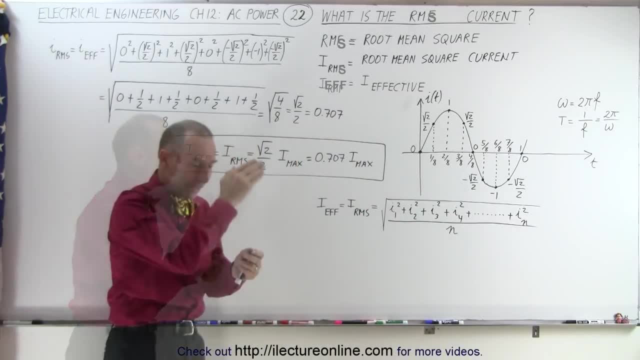 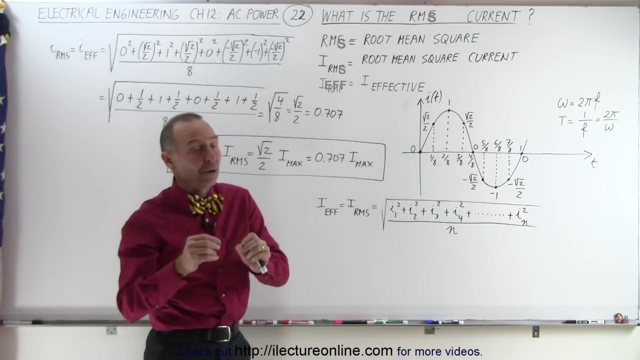 root, and hence the name, root mean square. We take the root of the mean of the squared values of the samples of the current. That's another way of saying that. And so now, of course, if we take eight samples, we may not get the exact root mean square value. It just happens so that it 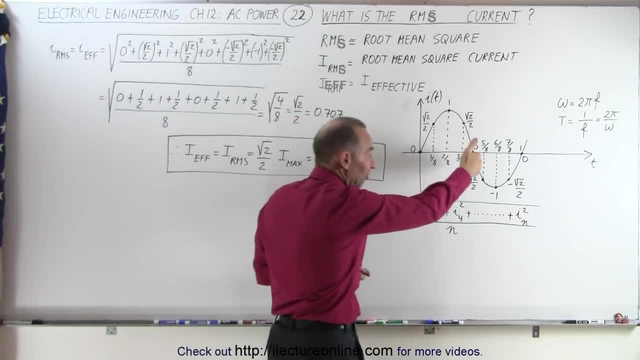 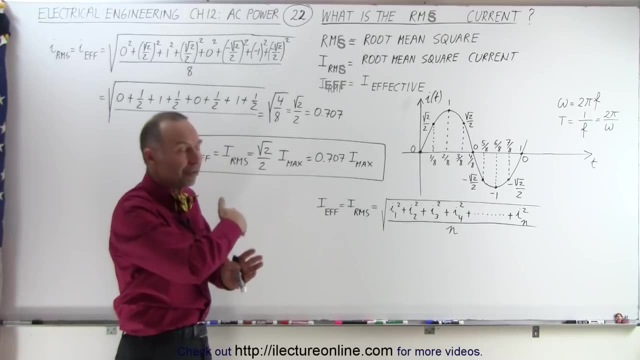 works out exactly here, But essentially, what you want to do is you want to take more samples. You want to take a hundred or a thousand or a million or a billion or an infinite number of samples. Of course, when you take an infinite number of samples- now we're talking about using the 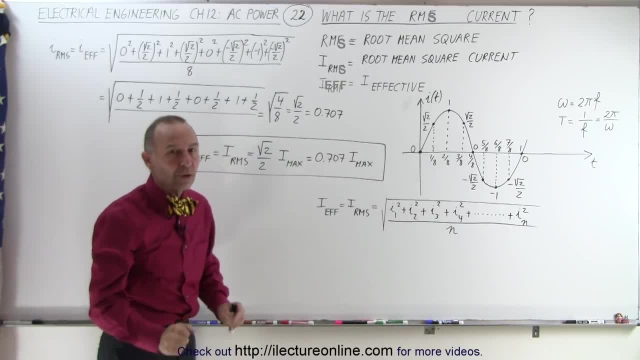 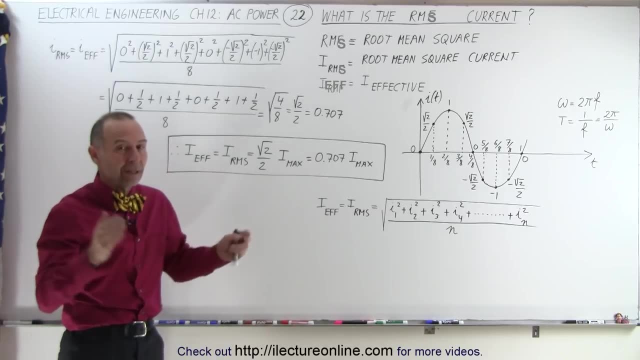 integration instead of the summation of n number of points. If we then use the integration method, then we get the exact value of the root mean square. If you use the summation value with a limited number of points, you may not get the exact root mean square. You may get something.